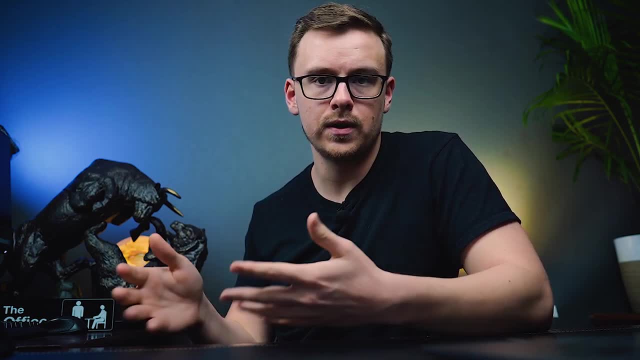 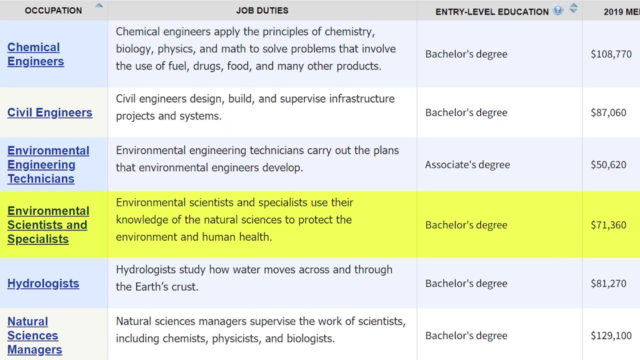 an hour And there's a few other career paths you might find yourself going down, so I'll just go ahead and list them off really quickly: Chemical engineer, civil engineer, environmental engineering technician, environmental scientist, hydrologist and natural sciences manager And, as you can see, the salary for all of them is relatively good and I always recommend, just to maximize your happiness, that you try to go for around seventy to eighty thousand dollars a year. I know that everybody's different and you know you might live in a part of the country where things are more. 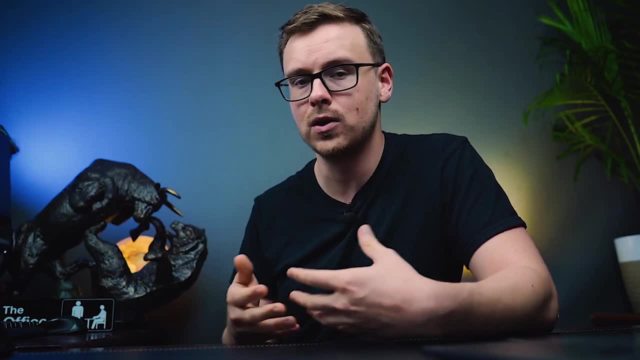 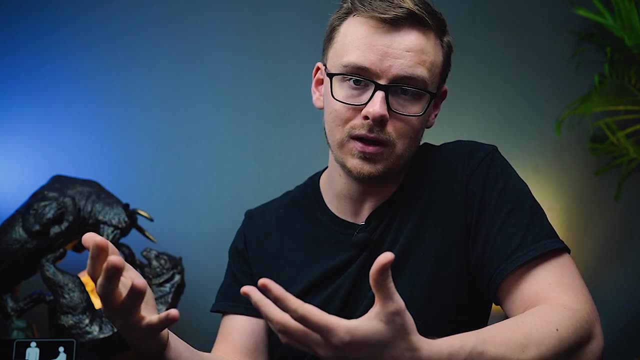 expensive, or maybe you're a minimalist and you can live off like twenty thousand dollars a year, but generally speaking, studies have shown that happiness is in fact going to increase the more money you make, up until a certain point, and that's usually around seventy to eighty thousand Now, if 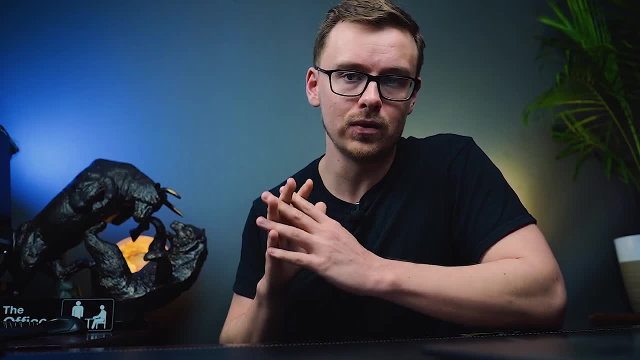 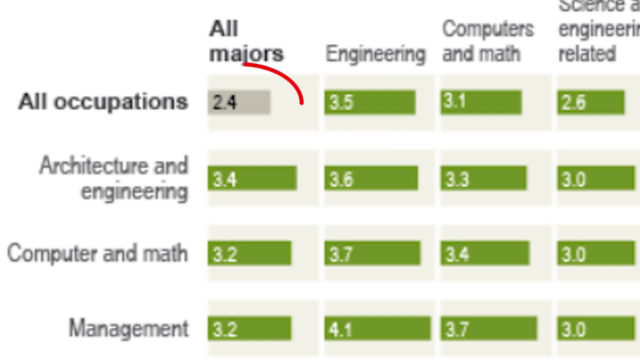 you look at the latest census and you see how much engineering degrees make over a lifetime. it is excellent By far. the number of people who graduate with a degree in engineering is going to be number one degree at around three point five million, compared to all the other ones which are: 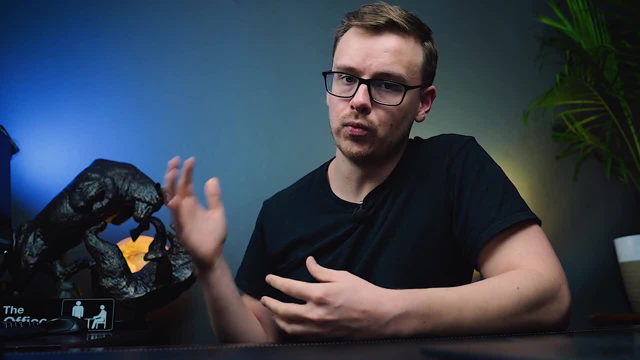 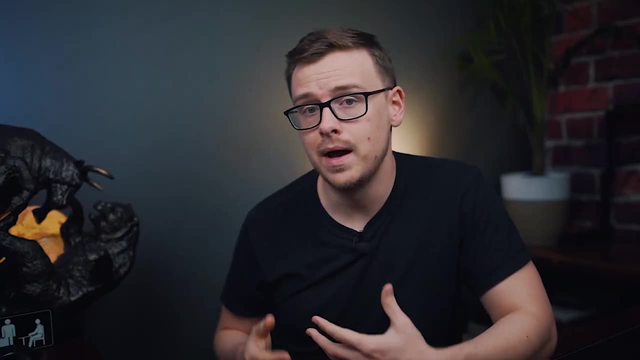 two point four. So it's no surprise here. engineering degrees score really well when it comes to salary or earning potential. I'm going to give this one a nine out of ten. Next, we're going to be talking about the most subjective section, which is satisfaction, and I like to break this one down. 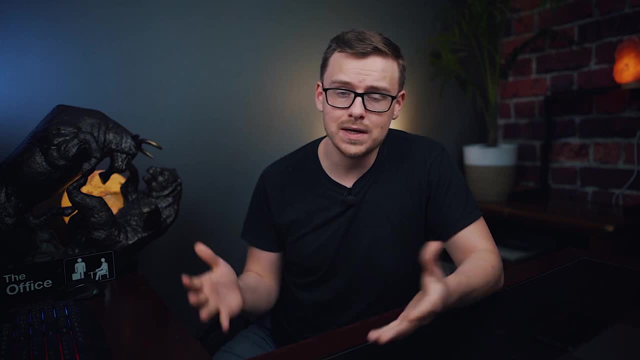 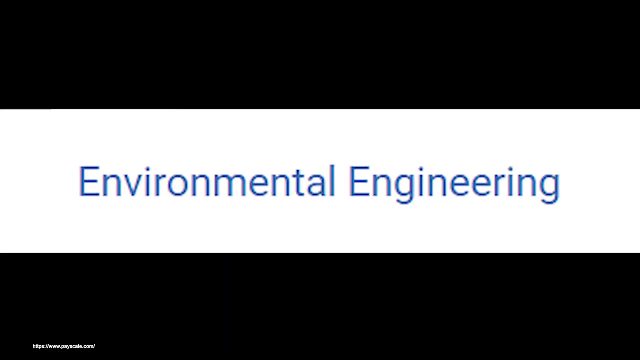 into meaning and job satisfaction, And meaning is basically how much you think your job positively impacts the rest of the world in a significant way. So for this degree it has a meaning score of about sixty four percent and if you compare that to one, that's really high and one. 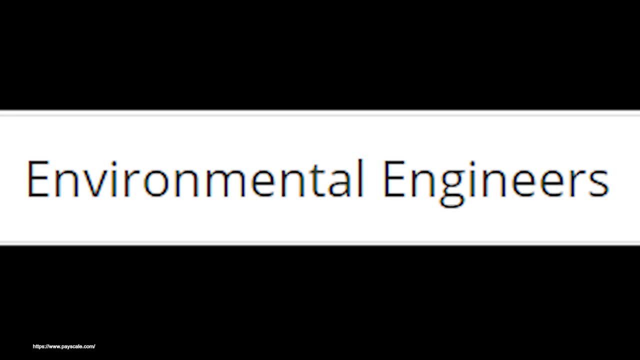 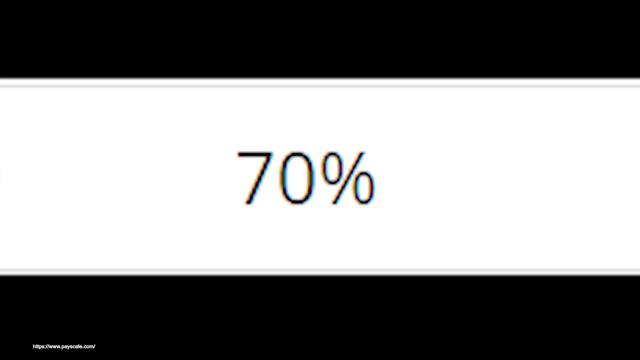 that's really low. you'll see that it's above average. Now, if you were to become an environmental engineer, the meaning score is seventy percent, which again is going to be above average, And if you look at the job satisfaction score, it's seventy two percent and you can compare that to a really 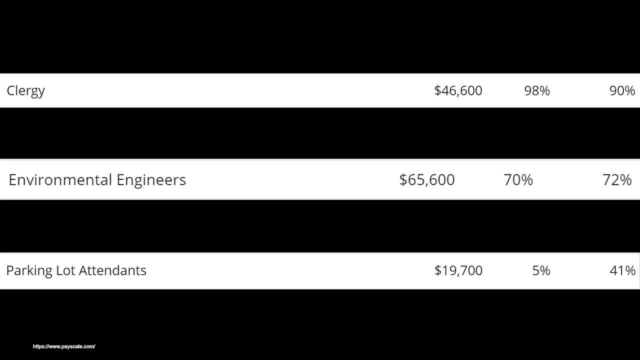 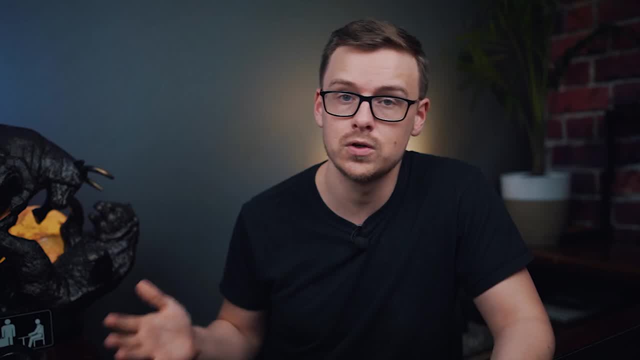 good one and a really bad one, And again it's going to be on the higher side, So everything is looking really good there. It looks like people who go into this career path not only find it meaningful, but they enjoy doing their job on a day to day basis. 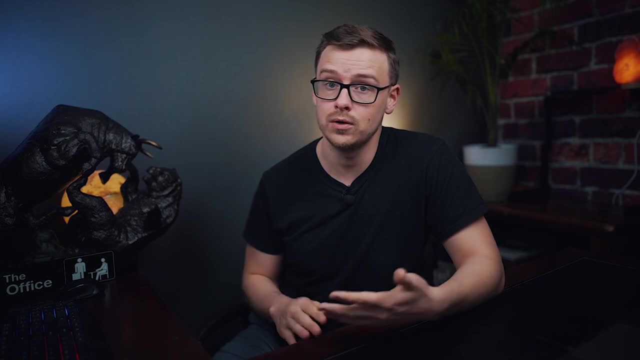 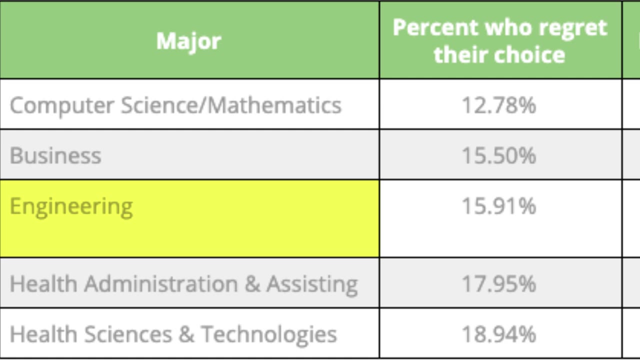 Now, another thing I like to look at is the percentage of people who regret getting their college degree, And ZipRecruiter released data and it shows that engineering is the third least regretted type of degree. Only around fifteen percent of people who got it regretted it, And 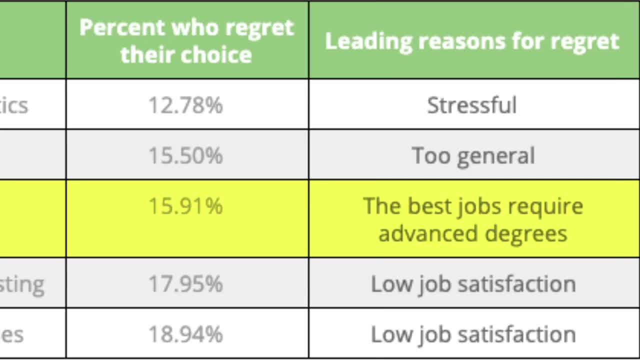 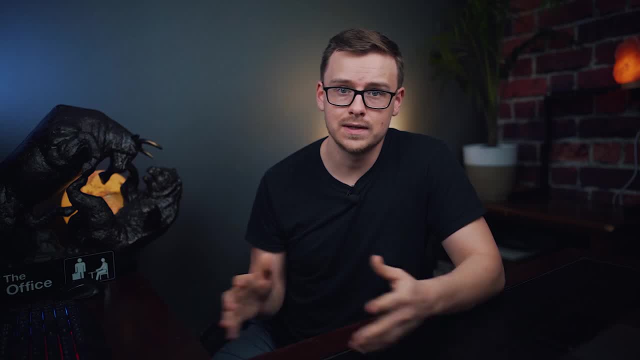 the main reason is because the best jobs out there sometimes require an advanced degree like a master's or a doctorate, But overall really good. This section is extremely subjective. Like I said, there's so many other things that can influence how you enjoy your job or how much meaning you. 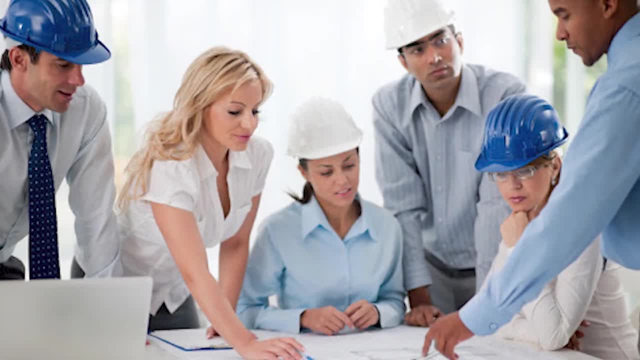 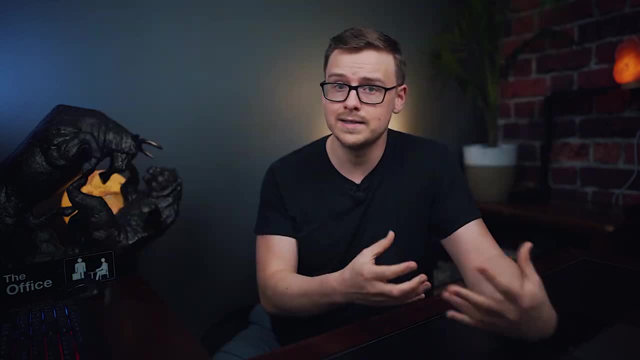 find in your job. It can influence how you feel about your job. It can influence how much you can be the people. you work with the company. you work for industry, you work in all kinds of different things where you live. For some people, salary is going to be very important if they have a high. 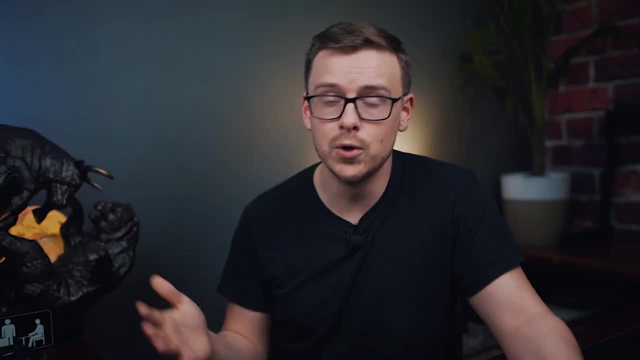 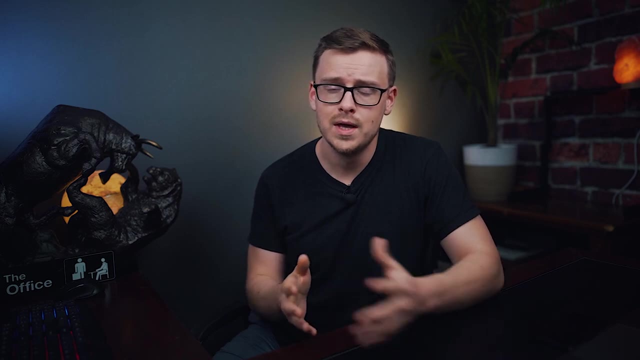 salary that will make them happy. For others it doesn't really matter. For most people it matters up to a certain point. So this is extremely subjective. for one person It could be amazing, for another person It could be awful, But overall I'm going to give this one a nine out of 10 when it 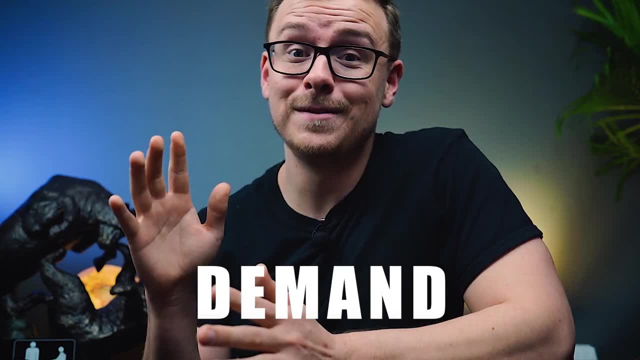 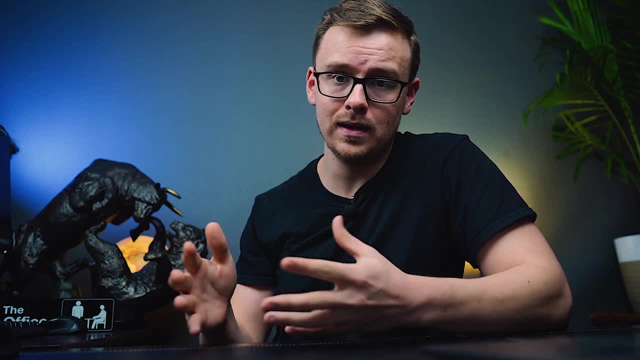 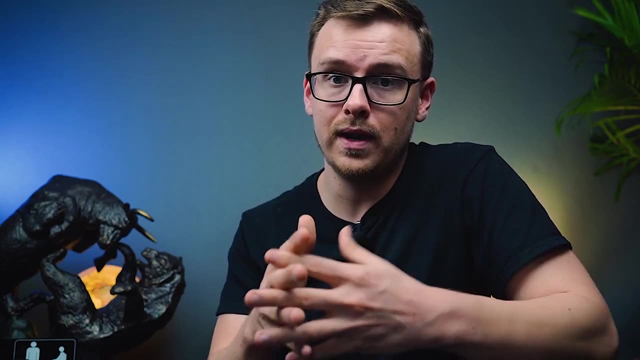 The reason for this is because everything else comes from demand. At the end of the day, the economy works in a supply and demand format. If you have skills that are in demand and there's not a lot of other people out there that have those skills, that can supply those skills, then they'll probably end up paying you more, They'll probably end up treating you better, and there's just going to be a lot more opportunity in general. So, when it comes to an environmental engineering career, there's 55,000 jobs available right now, and it's growing at 3%, which is as fast as average. 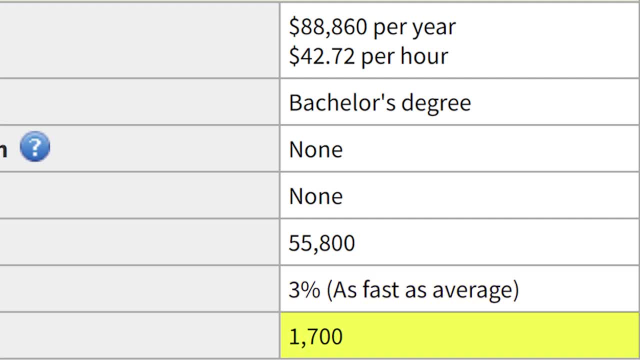 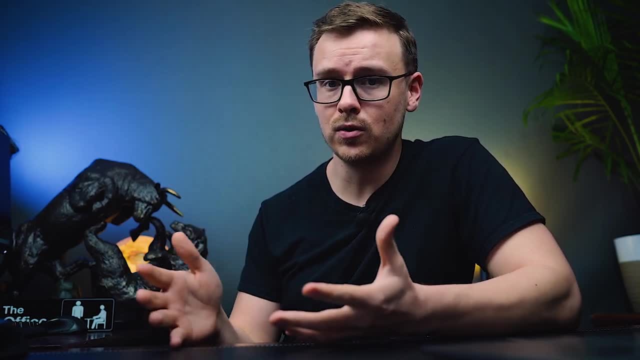 Meaning, over the next 10 years, you're going to have a lot more jobs available and you're going to have 1,700 new jobs created. To be honest with you, that's pretty average, not very impressive, and one of the downsides of getting an environmental engineering degree is it's not 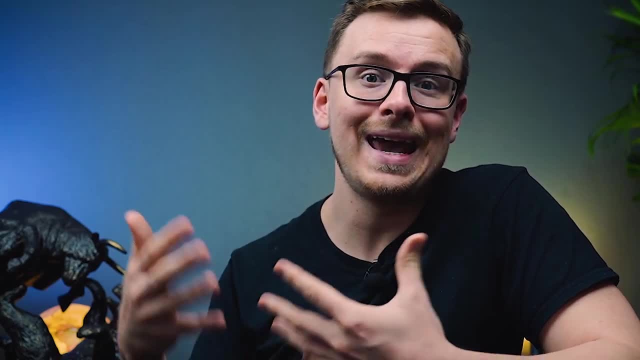 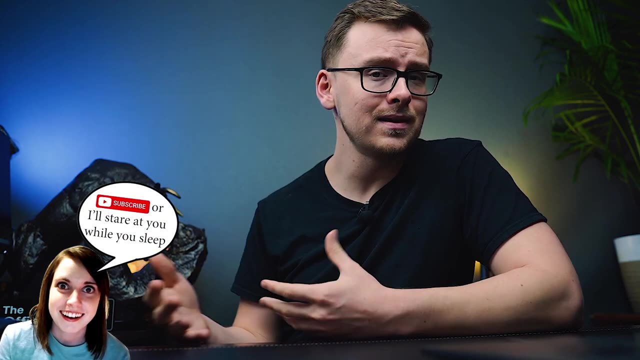 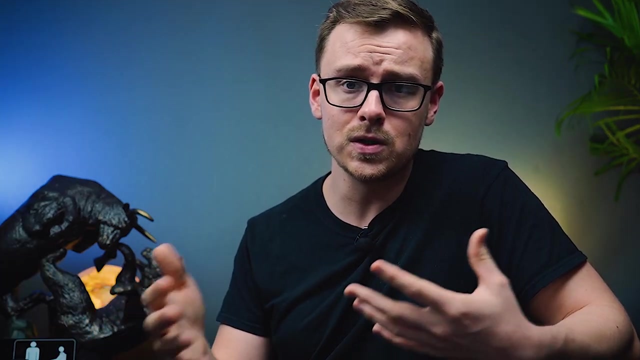 going to be as flexible as other types of engineering degrees, like mechanical engineering for instance. So, realistically speaking, with a mechanical or a chemical engineering degree you could do a lot of the same jobs as an environmental engineer, but it doesn't necessarily work in the other direction. A lot of the time, hiring managers and business owners are really used to mechanical. engineers applying for jobs, even if those jobs don't necessarily have much to do with engineering itself. A lot of the time, they'll end up hiring people with these degrees just because they respect them and they know that they're hiring somebody who's probably really smart and also really hard. 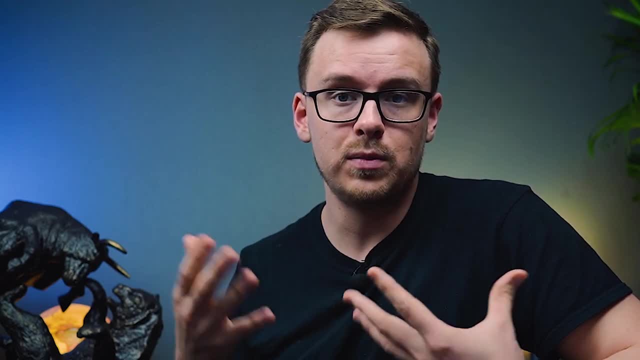 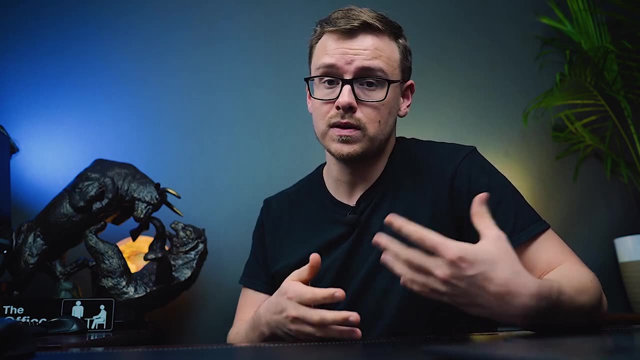 working, So it's almost like they have a little bit of real estate inside of people's heads who make important decisions when it comes to hiring. However, environmental engineering, although it might be just as good in terms of the skills you learn, isn't nearly as well known, and probably not. 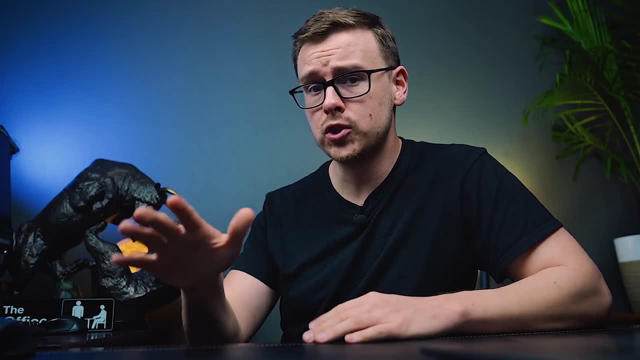 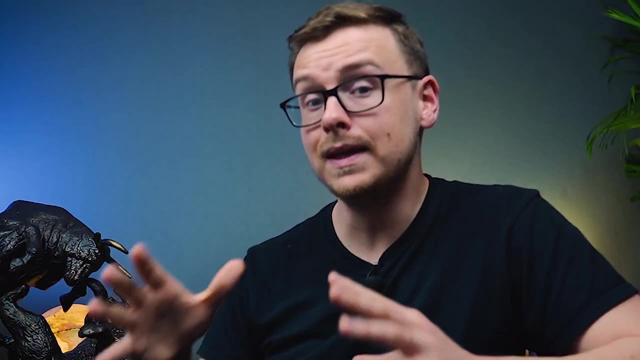 nearly as respected. So it could be much more difficult for you to get an environmental engineering degree, get your first job, especially if you aren't able to get a job as an environmental engineer Now. one way you can test the waters a little bit is to look up the keyword for the degree you're going. 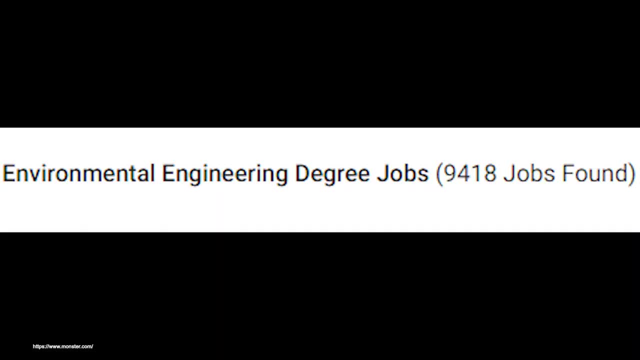 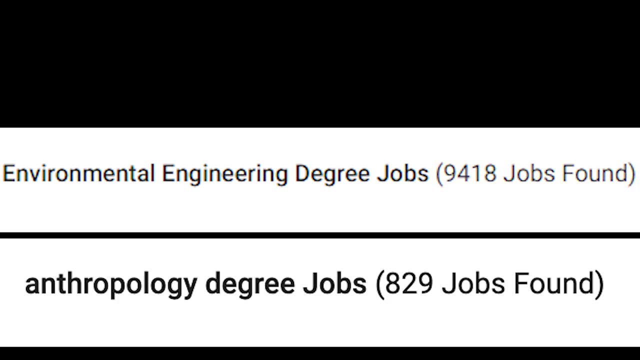 for on monstercom or indeedcom. So, for instance, you could type in environmental engineering degree and when I did that, 9,400 jobs popped up. You can compare that to a really bad one and a really good one and you'll see that it's actually not that bad. It's on the better side, especially when you 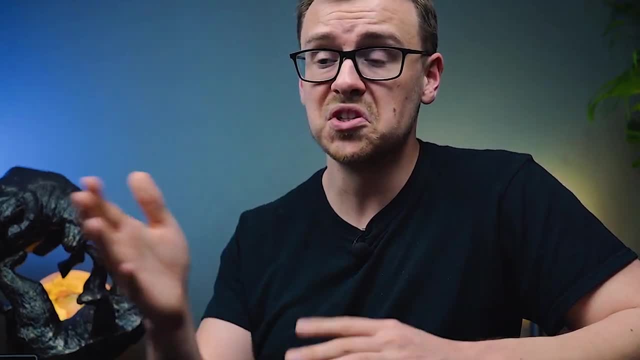 consider that not that many people are graduating with a degree every year. This is a pretty good sign. Now, in order to get your first job, you need to be able to get a job as an environmental engineer. Another thing that's really great about engineering degrees is when big companies 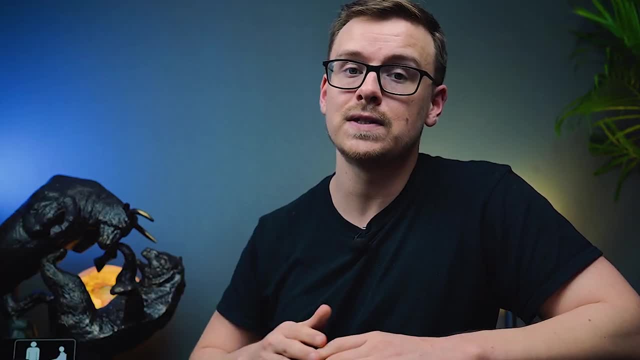 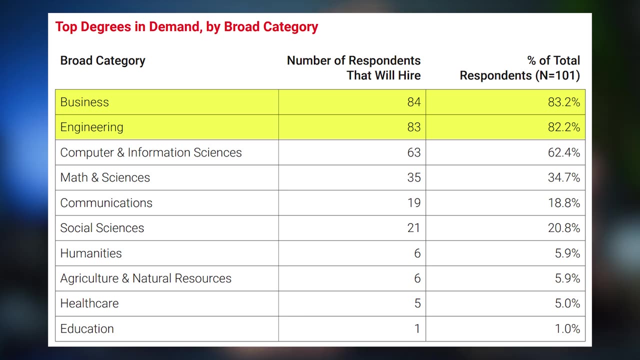 you know, fortune 500 companies are surveyed a lot of the time. they say that they love hiring engineers. It's usually either the first or the second most popular type of degree for those companies to hire, and business is up there as well. However, a lot of the time they're going to 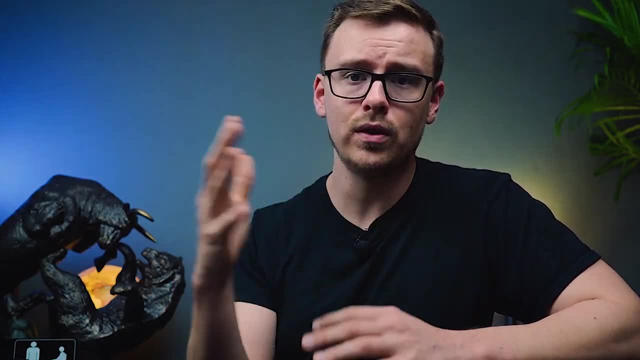 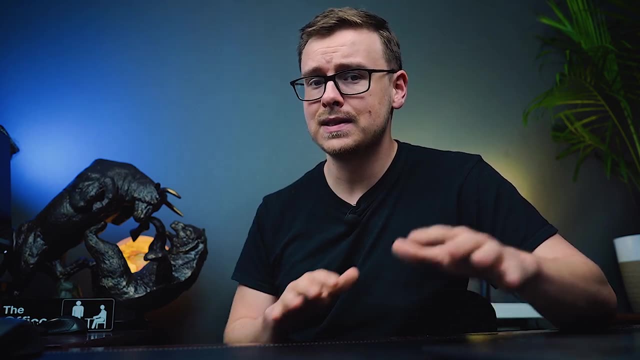 be looking for mechanical engineers- chemical, electrical, that sort of thing- because they're not nearly as familiar with this type of engineering major. So overall this degree is a little lacking in this category. Maybe it'll be different 20 years from now. I'm not sure, I don't know. 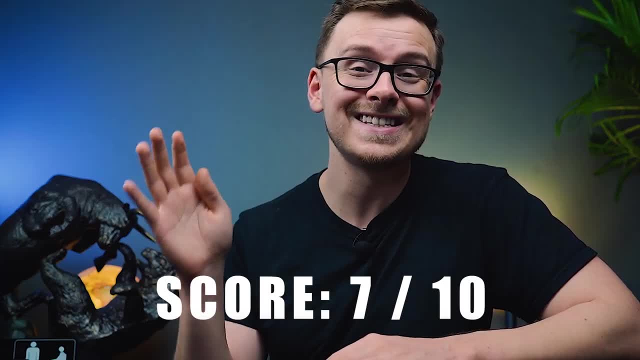 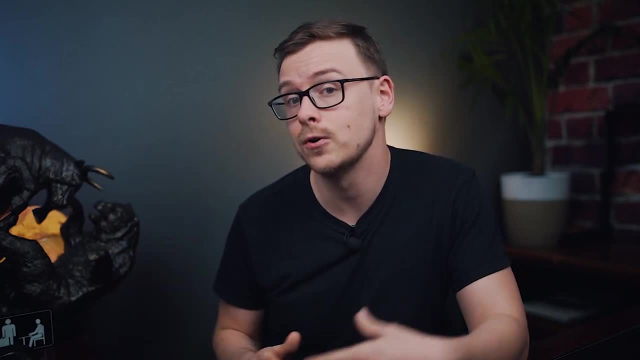 But right now I'm going to have to give this one a 7 out of 10.. Next, we're going to be talking about x-factors. This is anything else that I think is important that didn't make it into any of the other categories, So one thing I always like to mention when it comes to engineering degrees is: 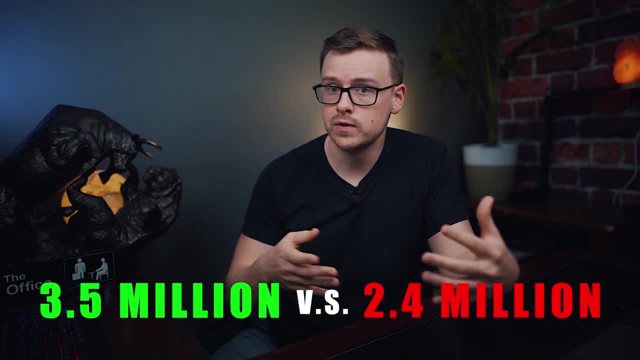 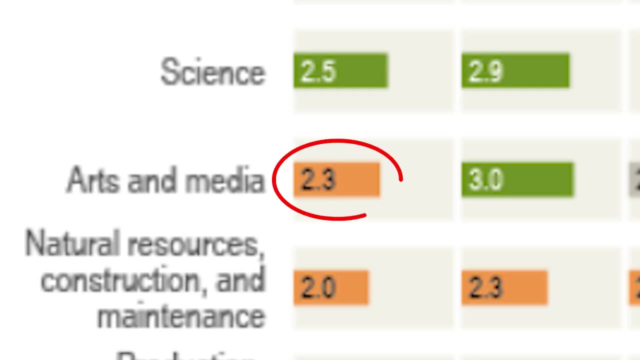 not only do you make more money over a lifetime- 3.5 million versus 2.4 million- but it's good pretty much no matter what career path you end up going down. So the average artist is going to make around 2.3 million over a lifetime, whereas the engineer that becomes an artist is going to make. 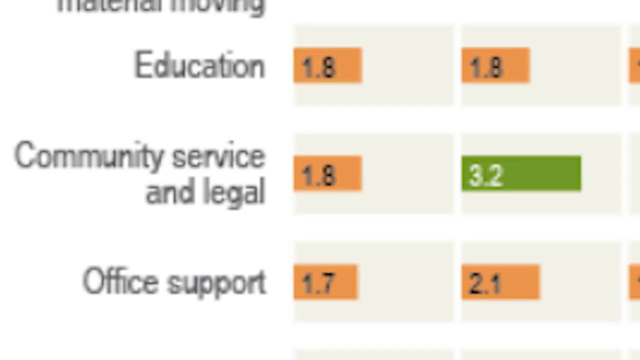 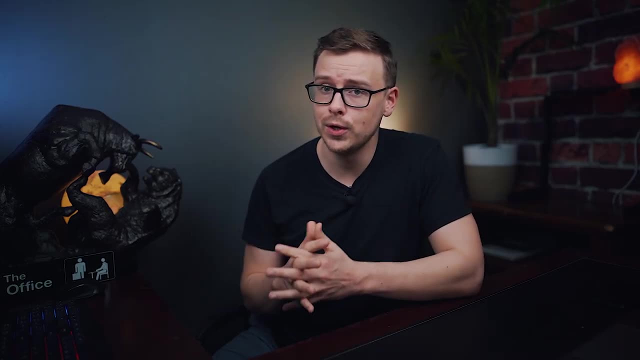 around 3 million. That is a huge difference. Same thing when it comes to community and legal services: It's going to be 1.8 versus 3.2 million. Engineering degree graduates tend to do really well, no matter what career path they end up going down, And there could be a multitude of reasons. 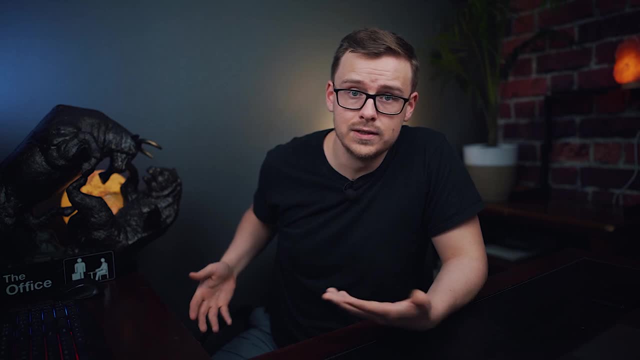 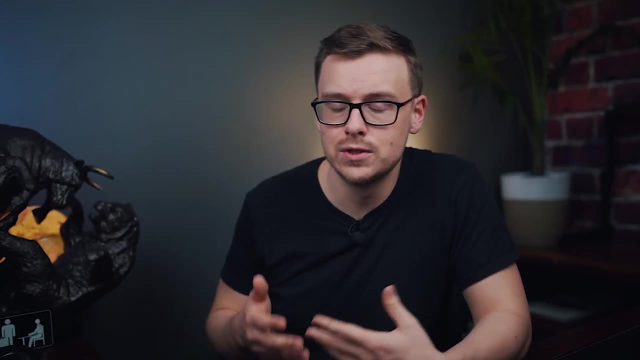 for this, but overall it is a good sign. Now, another thing I like to do is look up the skill index for these different types of careers and degrees, And you'll see that, of course, environmental engineering isn't going to show up on there, but something that's really close to it. 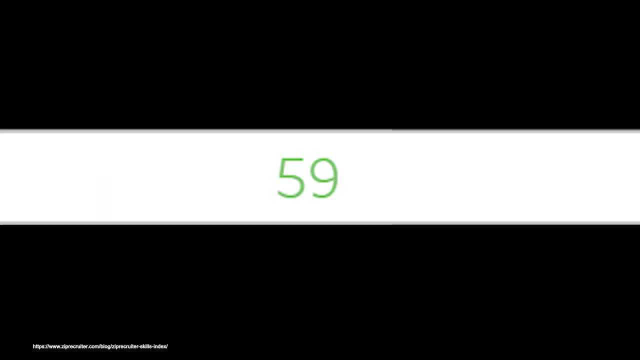 is going to be chemical engineering And that's going to be something that's going to show up on there. But something that's really close to it is going to be chemical engineering And that's one score is 59 out of 100.. You can compare that to the highest score and one of the lowest scores. 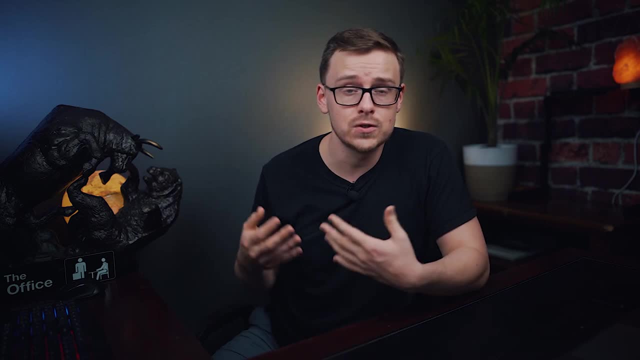 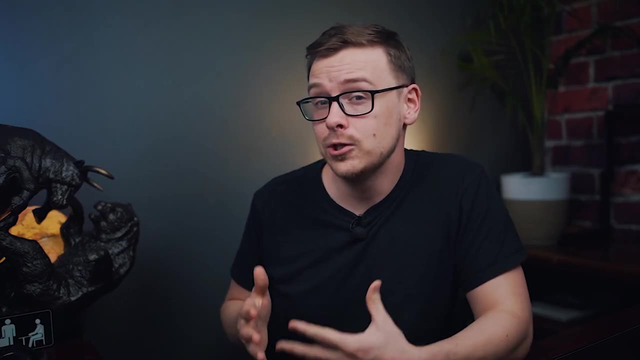 and you'll see that it's definitely on the higher side. That's a great sign, because it shows that hiring managers and business owners are looking for people who have these types of skills. Another thing I like to look at is the likelihood of automation, So, for instance, environmental 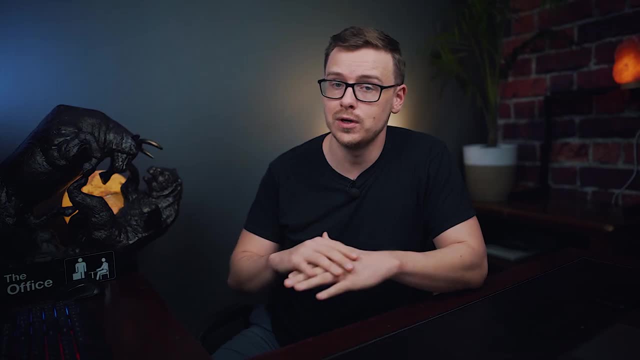 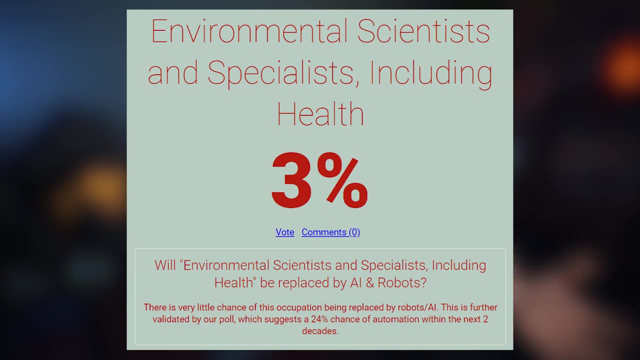 engineers have a 1.8% chance of automation, so pretty much it's not going to happen. Same thing with environmental scientists and specialists in general: about a 3% chance very, very low. And when it comes to outsourcing it's kind of the same thing. Usually engineers are relatively 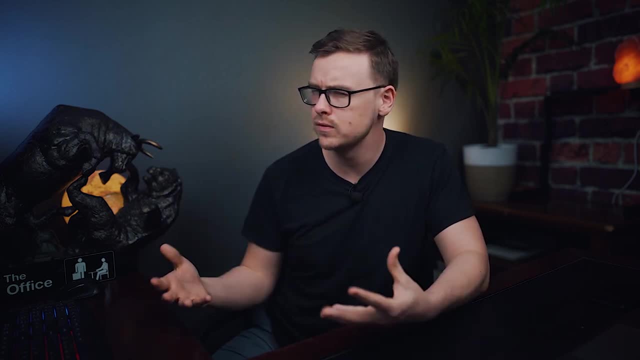 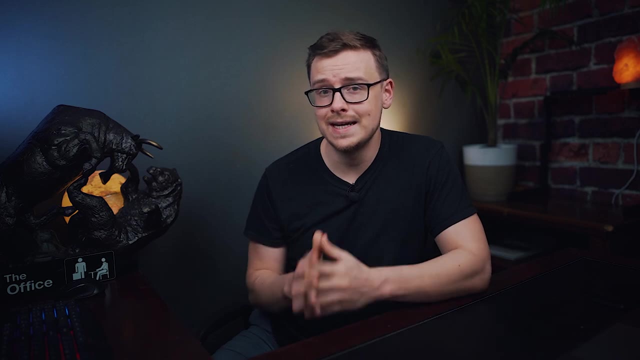 hands-on. They're going to be communicating with other people. There's a lot of creative intelligence involved, so very unlikely that it will be outsourced. Another thing I like to mention with engineering degrees in general is they tend to create a lot of millionaires and billionaires. 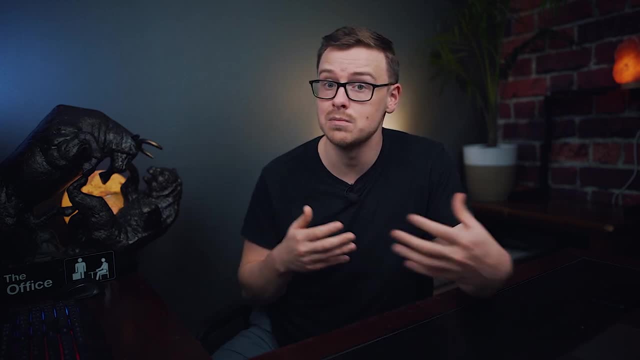 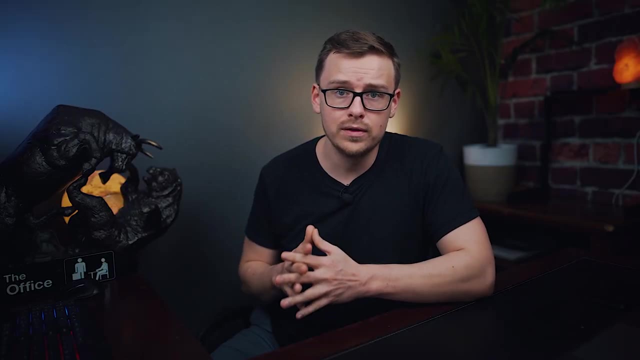 They're actually number one in terms of degrees. They create the most millionaires and billionaires, And the main reason for that, besides the high salary, is the fact that it is a really good segue into entrepreneurship. Engineers are the ultimate problem solver. 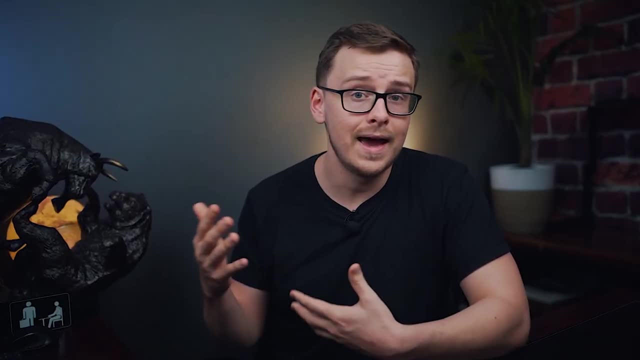 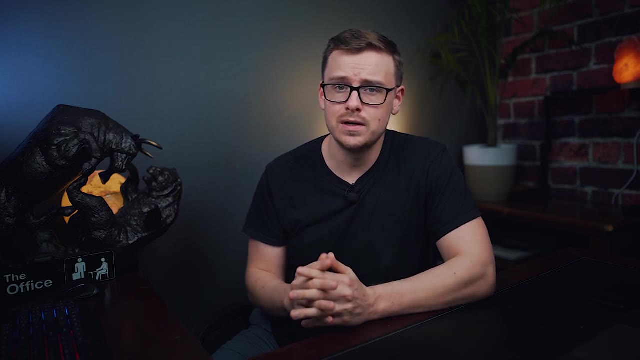 they are extremely practical when it comes to problem solving and, at the end of the day, that's what most of entrepreneurship is. That's basically 80% of it. So it's extremely flexible. With an engineering degree, you can go down so many different routes. You can work in almost. 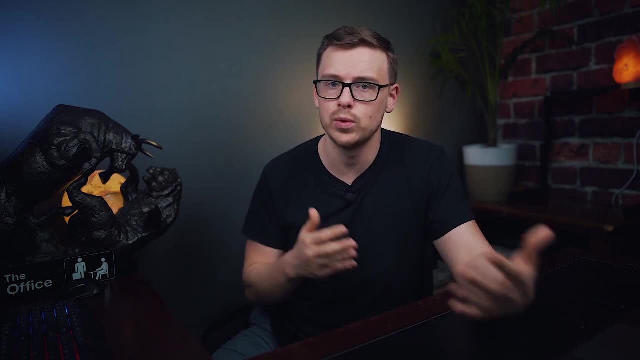 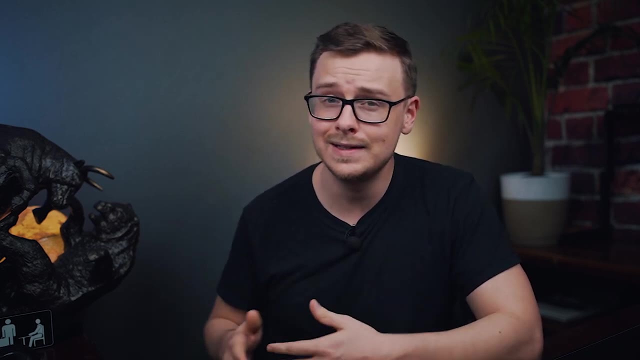 any industry and any business for all kinds of different careers. And then, once you've gotten a few years of experience, you've gotten some skills. you can go off on your own and start your own business and you'll likely have the technical skills to have a very good chance. 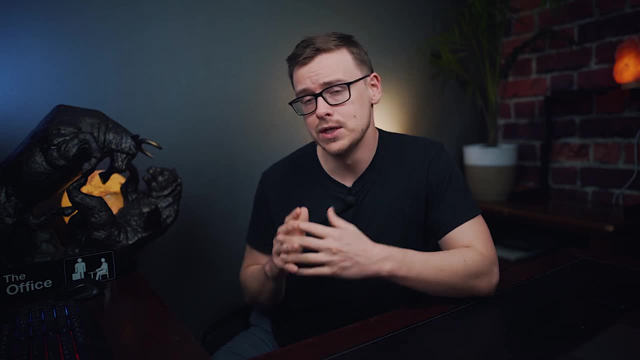 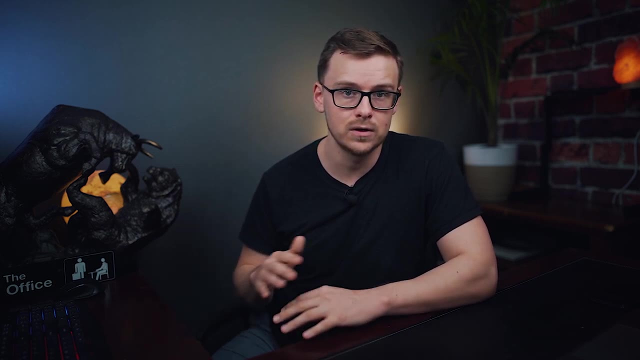 of being successful. Now, one last thing that I like to mention about engineering degrees is that they are very difficult. Okay, so you know. you want to know what you're getting yourself into. Engineering degrees are tough. you're going to be studying all the 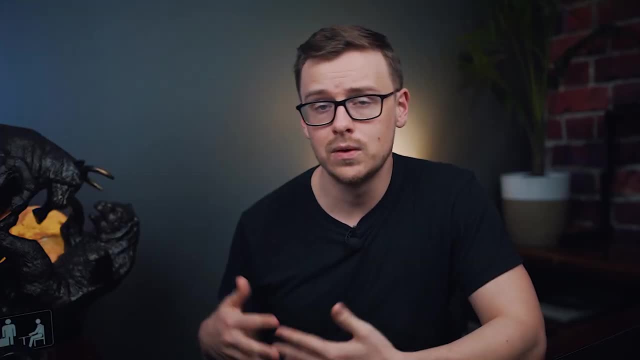 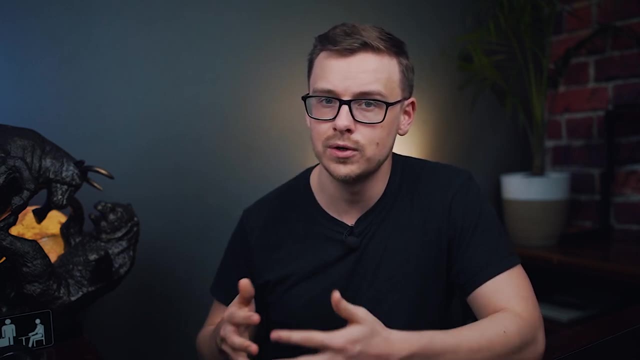 time it's going to be one of the hardest things you have to do, But, with that being said, when I was researching this video, a lot of people on forums said that it's not as hard as some of the other engineering degrees, and some of the skills you learn might not necessarily be as practical, or 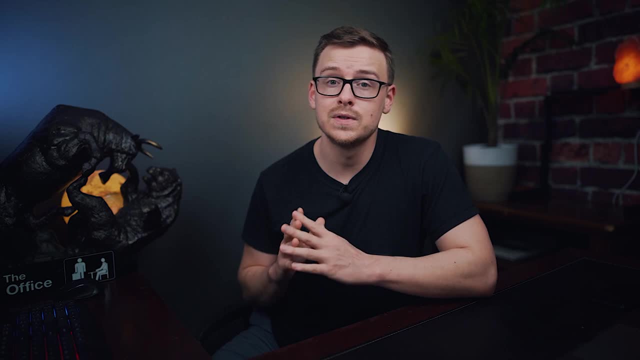 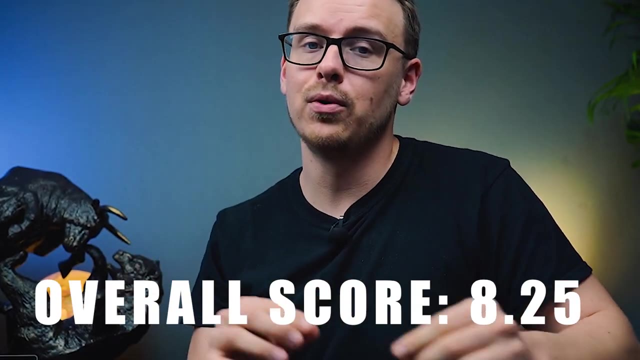 as applicable. So overall, when it comes to x-factors, I'm going to give this one an 8 out of 10.. So when you take all four of those and divide it by four, the final score is going to be 8.25 out. 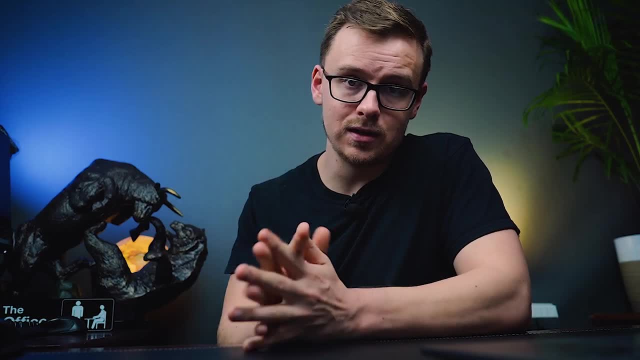 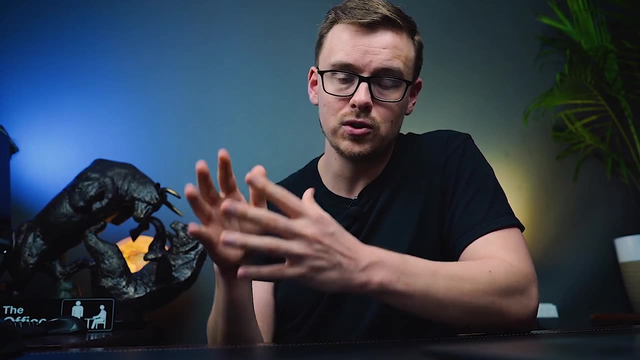 of 10.. That is pretty good. Now, of course, this is subjective. it's going to be different for everybody, so make sure that you do your research. I'm assuming here that you've done your due diligence, you've done your research, you've talked to people in the career path that you're trying to.